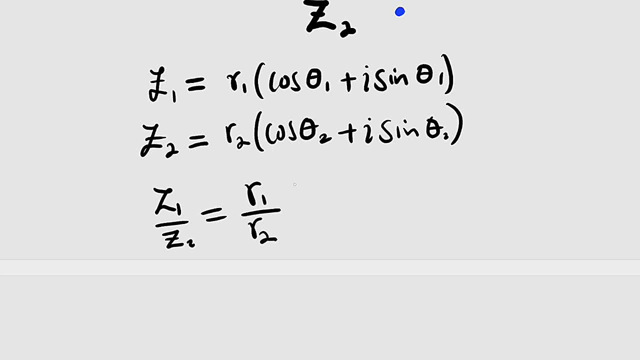 to r1 divided by r2, multiplied by cosine of theta1 minus theta2, then plus i sine of theta2, plus i sine of theta1 minus theta2.. So this is the formula we are going to apply in dealing with this problem. So first of all, let us transform each one of them into its polar form. We have 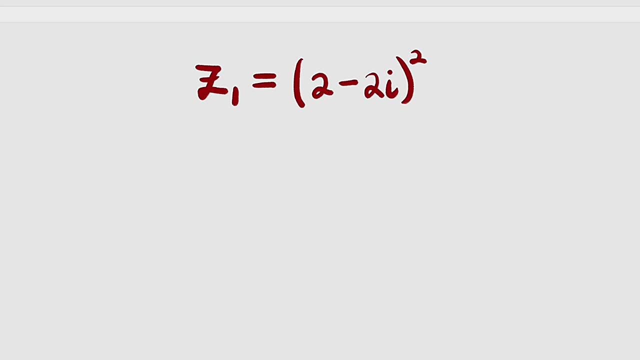 the first one here: z1 equal to 2 minus 2i to the power of 2.. What is r1?? That is the modulus. It is going to be the square root of the real part, which is 2 squared plus also the imaginary part. 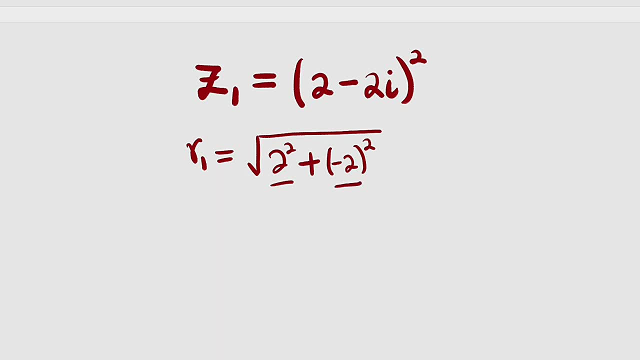 2. all squared, This is 4 plus 4 is equal to 8.. Square root of 8 is 2 root 2, right? So therefore, r1 is equal to 2 root 2.. And what about the angle theta? If you observe, this angle will be in the. 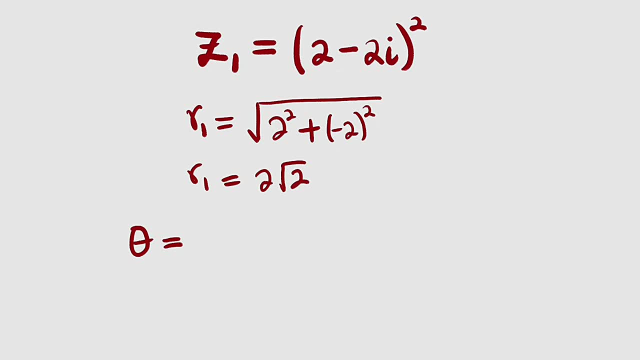 fourth quadrant because the real part is positive while the imaginary part is negative. So if you take first quadrant as reference, we are going to take all positive values. So you have to subtract the result from 360 degrees because we are in the fourth quadrant. So this is: 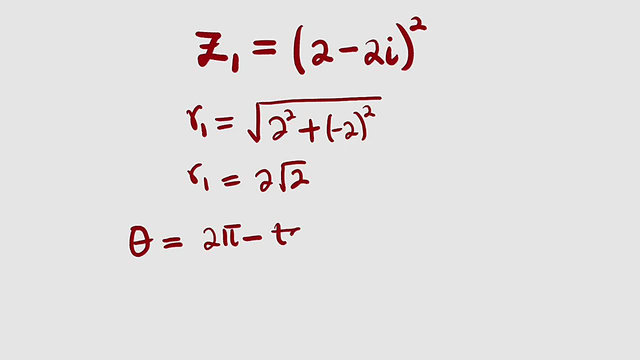 2pi, which is 360 minus tan inverse of what 2 divided by 2. That is imaginary part divided by the real part, And 2 divided by 2 is equal to 1.. Tan inverse of 1 is pi divided by 4.. So we have: 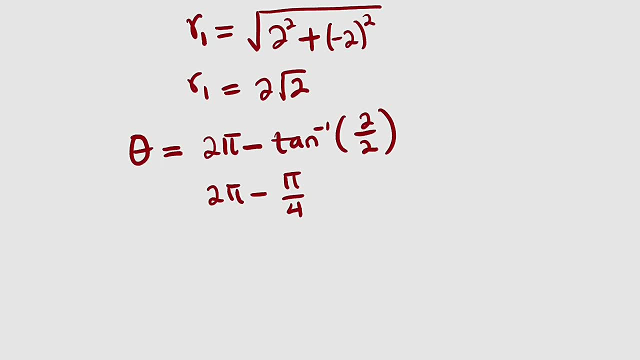 z2 times. z2 times this angle is equal to very smallELLER. We say: r1 is equal to 6 pi JavaScript plus 3, where everything is in a expandable state, 10 times 4, which is equal to 7 pi divided by. 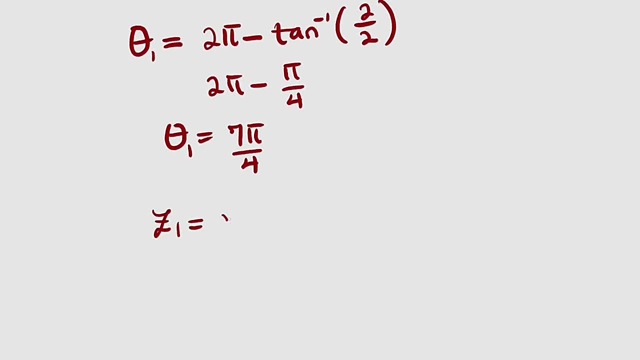 4, right? Therefore, our angle is equal to 7 pi divide by 4.. And this angle is theta 1, remember z1, equal to r1.. But what is r1? 2 root 2.. Then multiplied by cosine of theta 1, which is 7 pi, 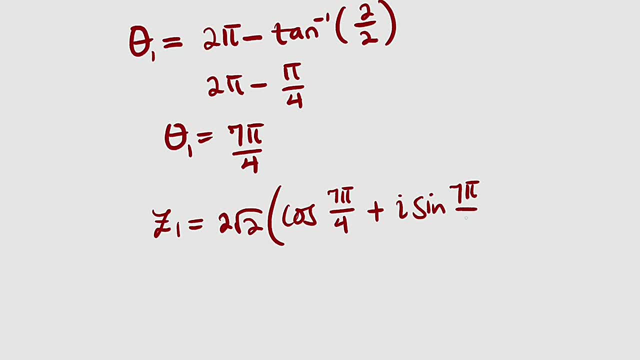 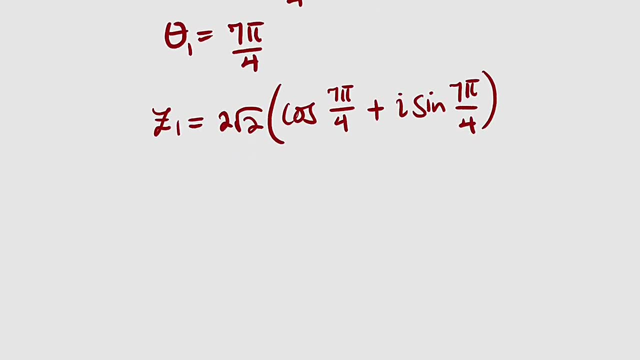 of 7 pi divided by 4. but remember, our complex number is to the power of 2, so we are going to square this: z1 squared is equal to R squared, then multiplied by, you also have to multiply the angle by that power, which is 2, so we have cosine. 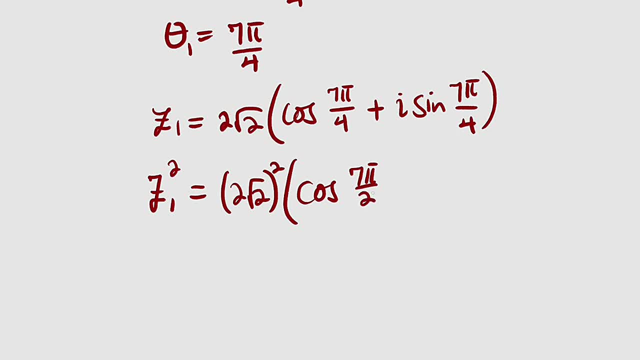 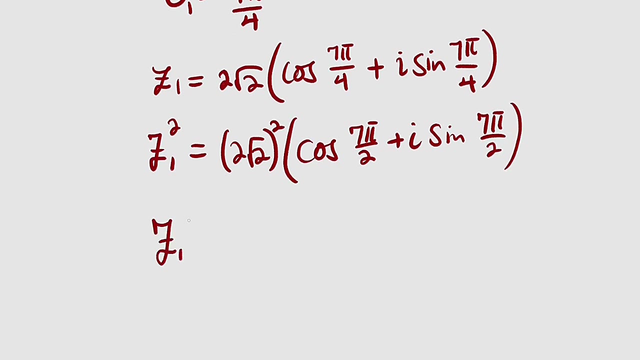 of what 7 pi divided by 2. if you multiply it by 2, 2 will go into 4, 2 times. then plus i sine of 7 pi divided by 2, z1 to the power of 2 is equal to. here we have: 2 squared is 4 and this is 2 4 times 2 is 8, so this is 8 multiplied. 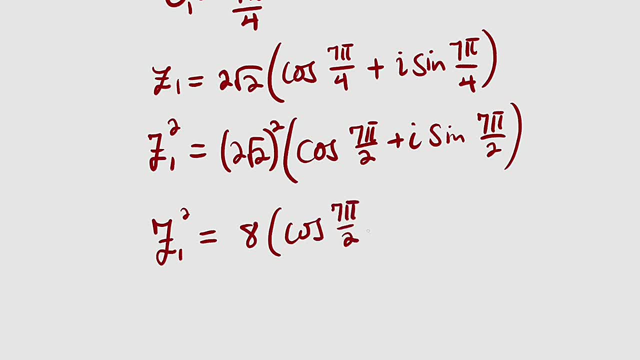 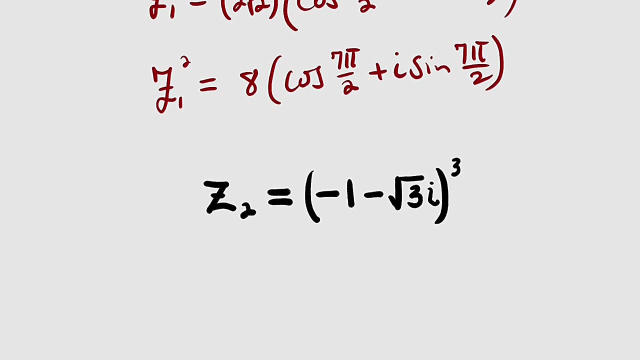 by cosine of 7 pi pi divided by 2, plus i sine of 7 pi divided by 2.. So we are done with the first complex number. Now let us take the second one. Here is the second complex number. We are going to find R2, which is equal to the square root of the real 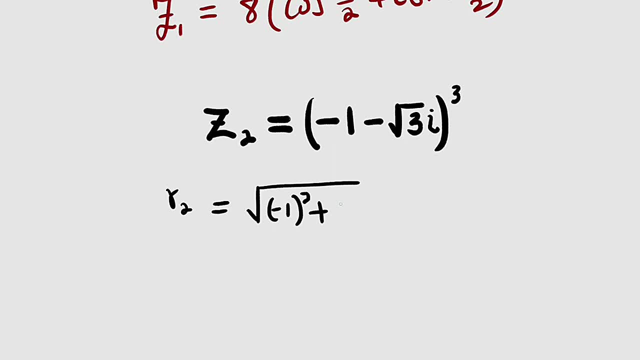 part squared, negative 1, all squared, plus the imaginary part negative root, 3, also squared, This is 1.. This is 3.. 1 plus 3 is 4.. Square root of 4 is 2.. Therefore, R2 is equal to 2.. What about the angle? If you observe, this is in the third quadrant. 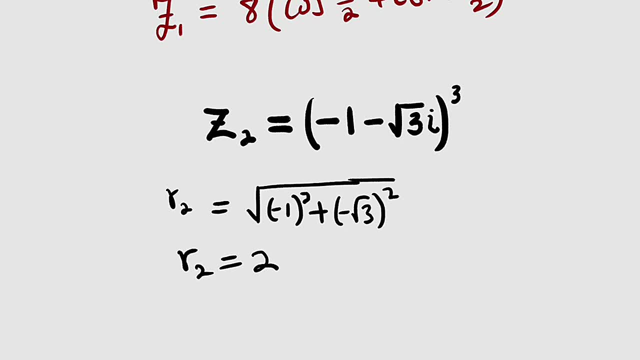 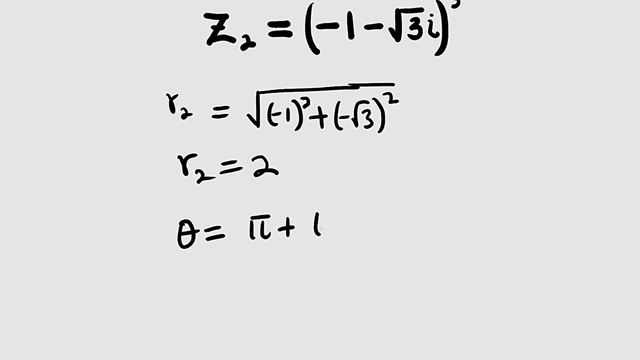 which is greater than 180.. So we are going to assume we are in the first quadrant, but whatever angle we obtain, we have to add it to 180 because it is greater than 180. Our angle will be equal to pi plus tan. inverse of what? 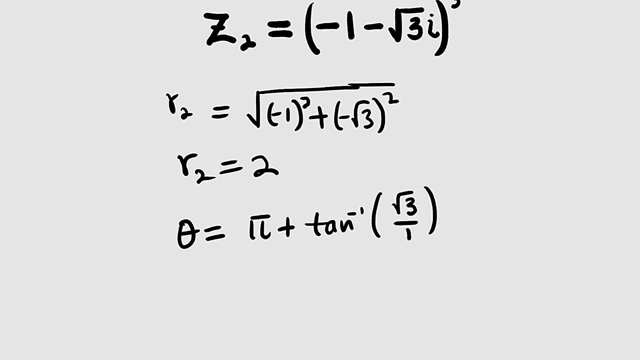 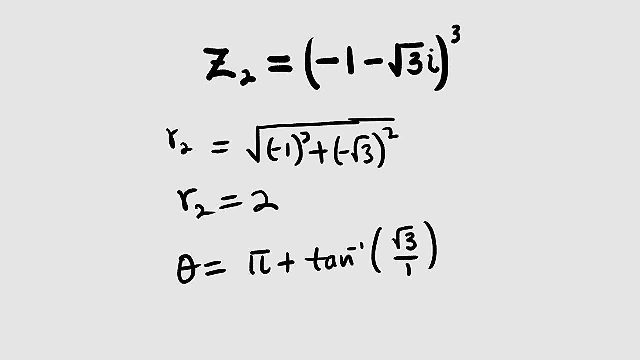 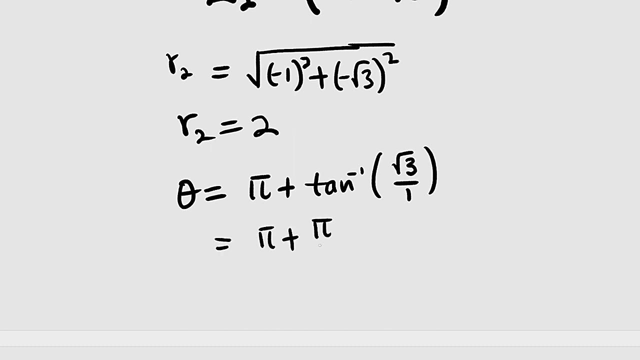 Root 3 divided by 1.. We are taking all positive values because we want to use the reference angle. Root 3 divided by 1 is root 3.. Tan inverse of root 3 is pi divided by 3.. So this is equal to pi plus pi divided by 3, which is equal to 4 pi. 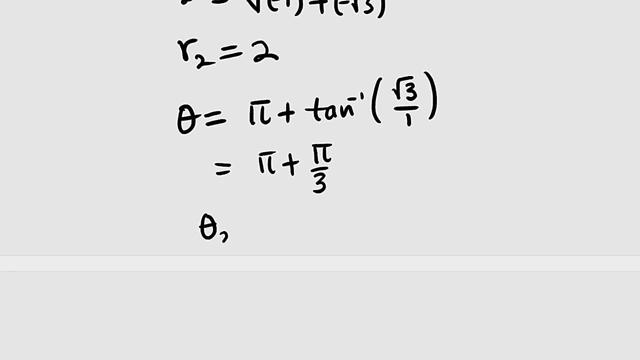 divided by 3, right? So our angle, which is theta 2, is equal to 4 pi divided by 3.. So what about our complex number? in its fuller form, z? 2 will be equal to R. What is our R? R is 2 function multiplied by cosine of the angle. which is 4 pi divided by 3, then plus I sine of 4 pi divided over equal r. So if this is equal to R, our R2 will be equal to r. If that is R, then we gotta compute. r means ji ∗θ will be equal to r. 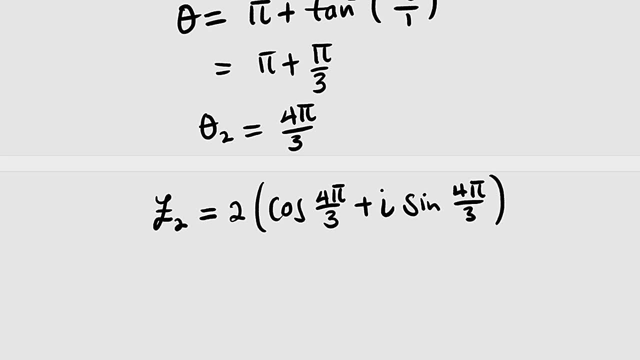 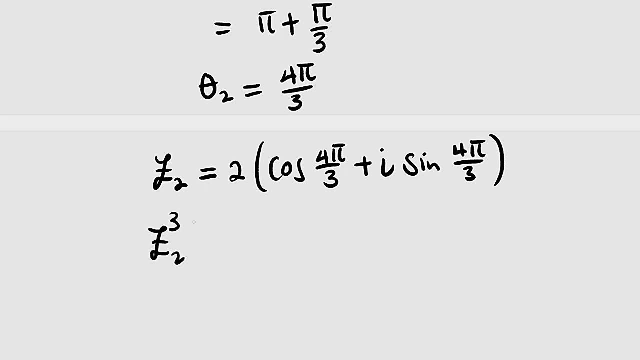 divide by 3, but remember our complex number is to the power of 3, so we are going to take it to the power of 3. z2 to the power of 3 is equal to 2 to the power of 3. then multiply by cosine of. 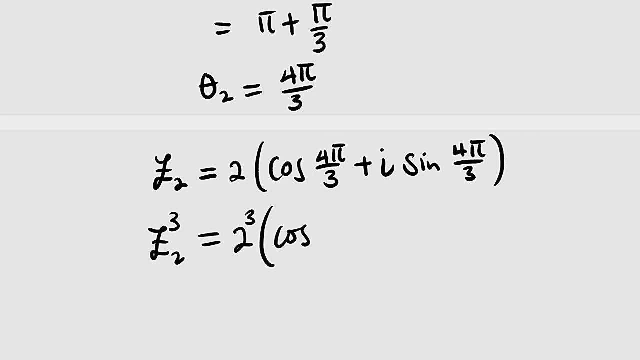 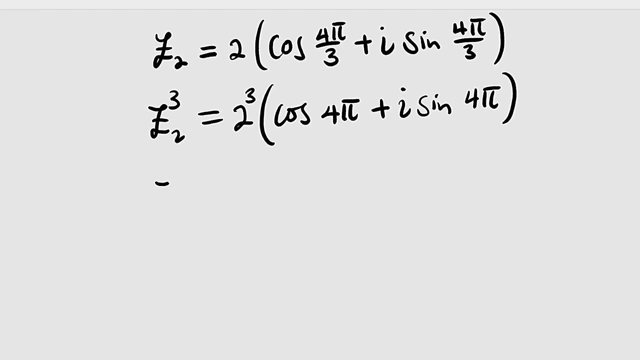 the angle, multiply by 3, 3 will cancel 3, leaving only 4 pi here. then plus i sine of what 4 pi. we are almost done. z2 to the power of 3 is equal to 8, multiplied by cosine of 4 pi, plus i sine of 4 pi. but remember, we are looking for what? 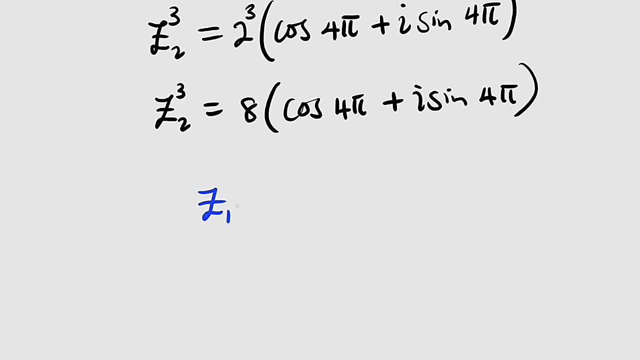 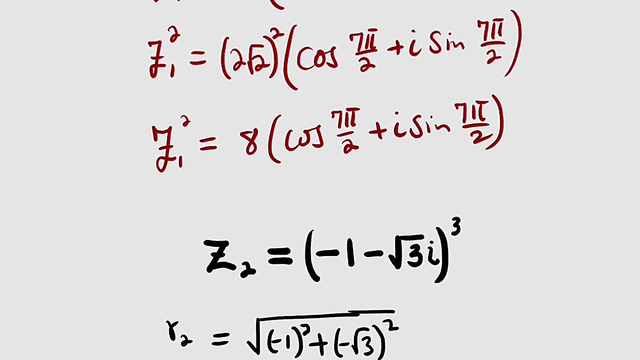 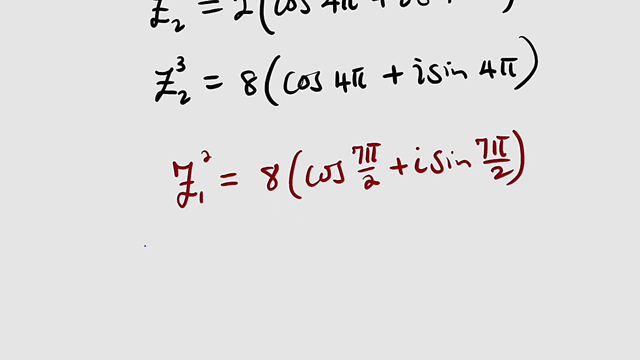 z 1 to the power of 2, divided by z2 to the power of 3, which is equal to you. divide their radius. they have the same radius this time around, right. 8, 8. let me even bring this one closer, so look at it here: z1 squared, divided by z2 to the power of 3, this is equal to. 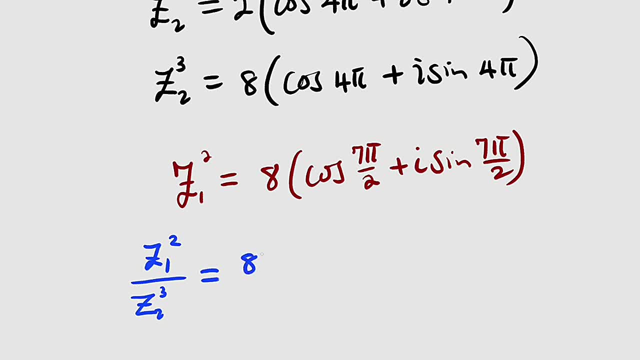 you divide by z2 to the power of 3, this is equal to you divide by z2 to the power of 3, with the location of this z1 right and now the whole system is of course altogether three. Hausch sporadicW 해도 to be zero. so I